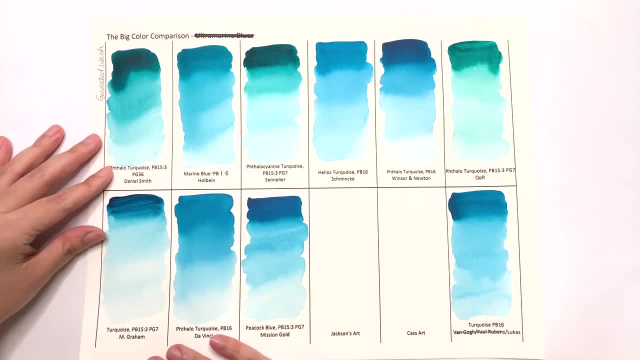 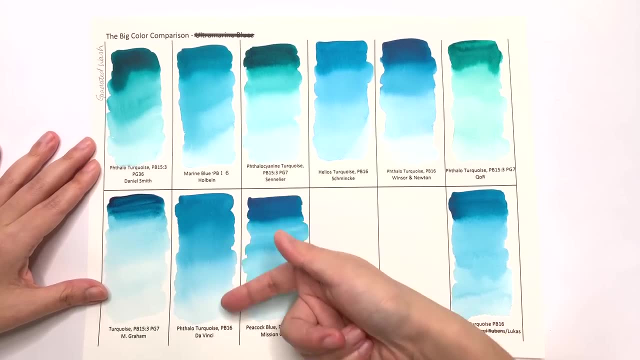 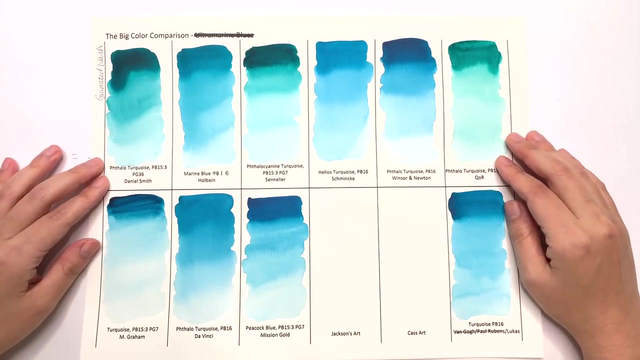 for both colors have just whooshed Across the page and you can almost see that speed in the colors because you get these very, very, very subtle lines going across, which kind of expresses the speed at which the pigments moved. So bravo to Da Vinci for being able to create such a smooth, gradated wash on a very, very economical 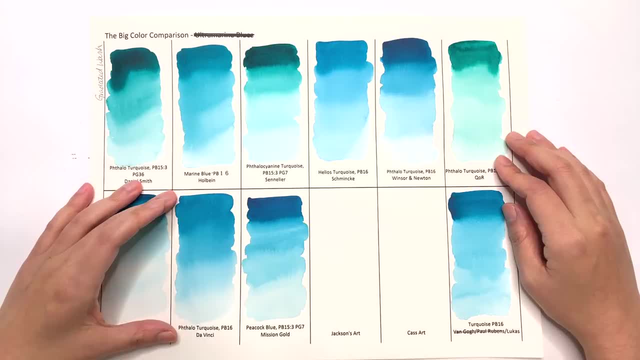 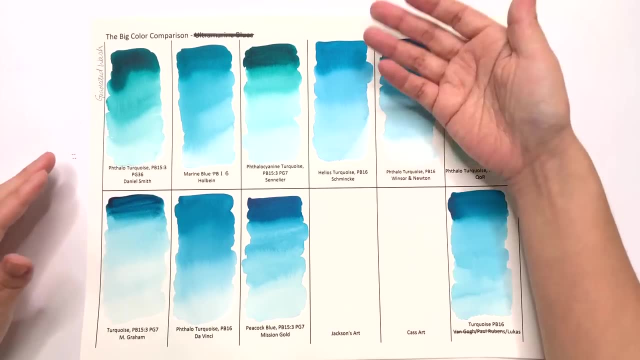 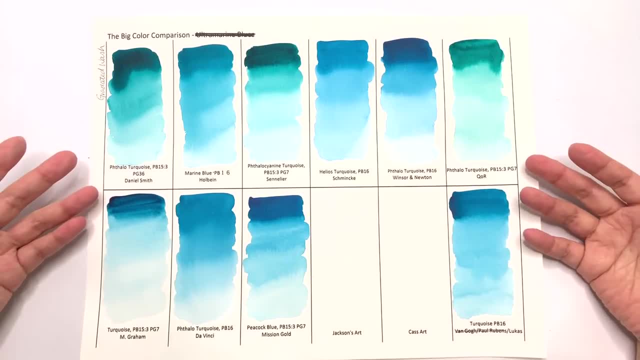 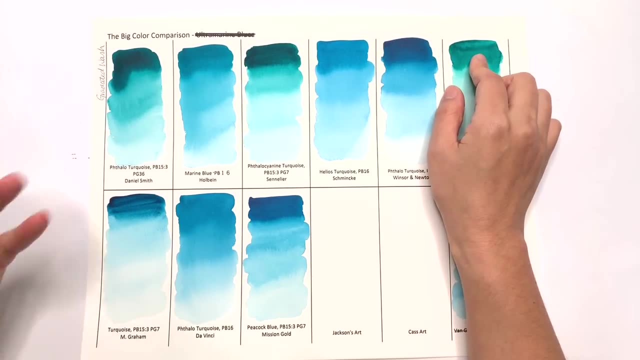 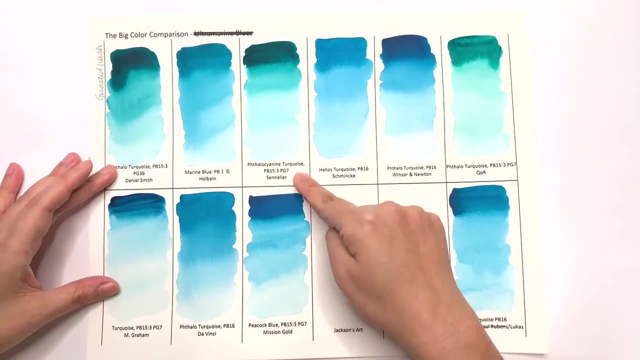 rest of the colors With the rest of the colors, the master, which is these colors at the top, where the colors are pretty concentrated with quite minimal amount of water, tend to stay up at the top And you can really see that in the Daniel Smith and Sennelier Mission. Gold and M. 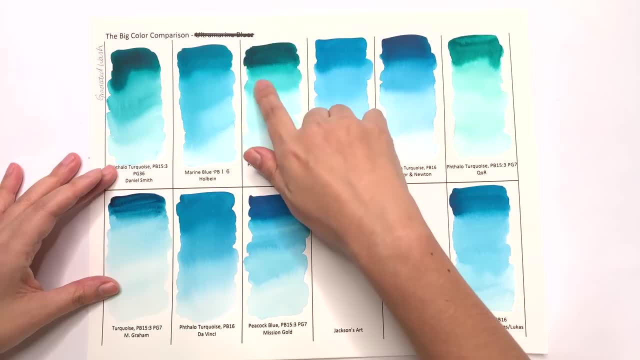 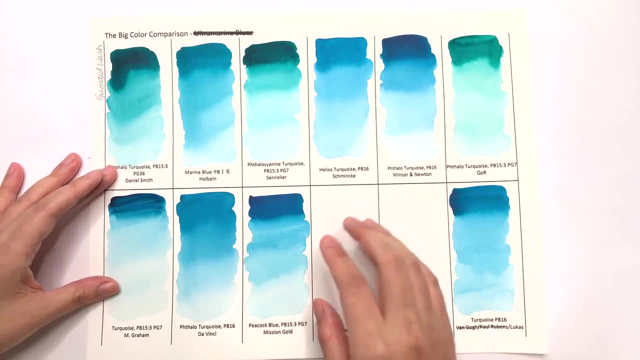 Graham. And then there's like a big step in how I think the next section is, whereas with the Da Vinci one it's very, very smooth. I would say the worst culprits at this is definitely M Graham, Daniel Smith, Sennelier. 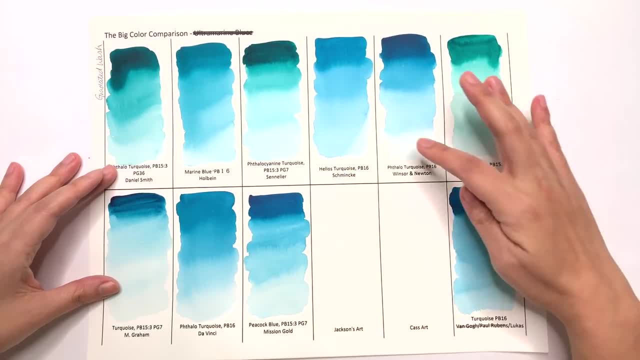 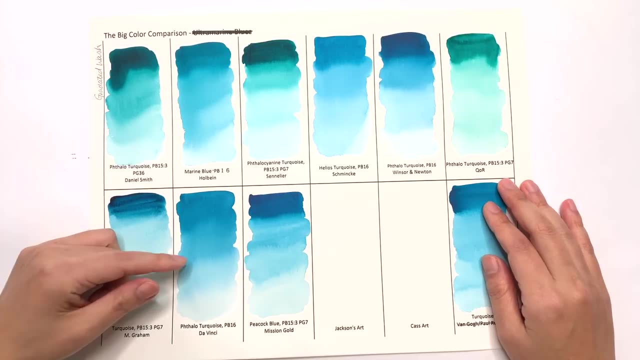 Mission Gold and Coir, surprisingly, with Winsor & Newton and Lucas being no bad at it. So if you do do a lot of gradated wash, do consider Da Vinci, Holbein or Schmincke before you consider all the other colors. 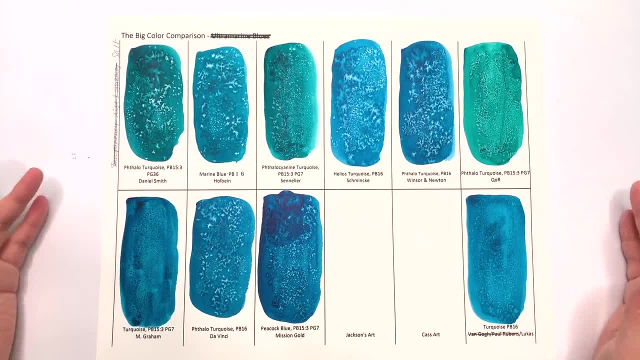 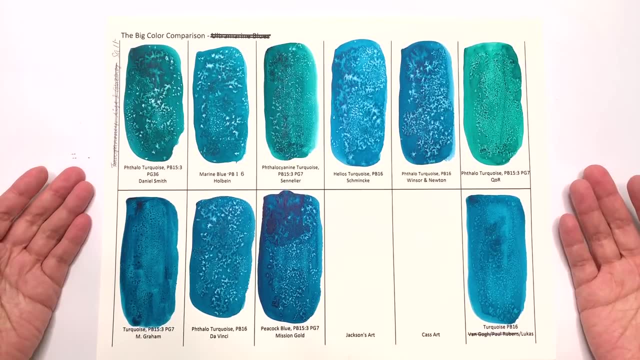 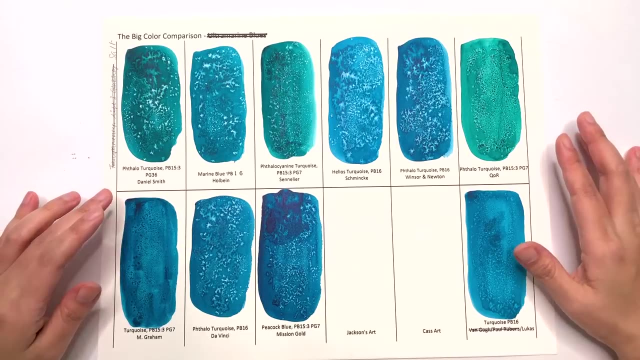 Now look at the salt test, Just like the salt test in Ultramarine, I am surprised to see the results of this test because the reactions were so varied- M Graham, Coir and Lucas. it basically did nothing, No reaction, particularly M Graham and Lucas Coir. you do see a little. 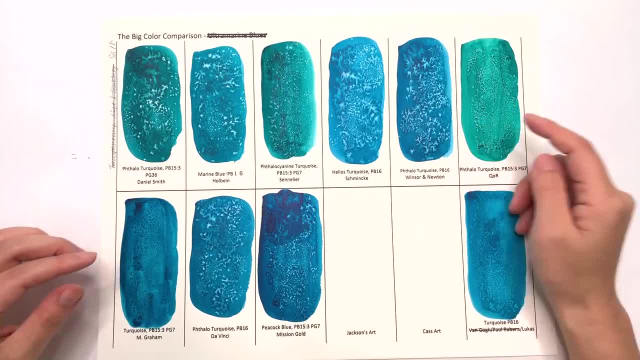 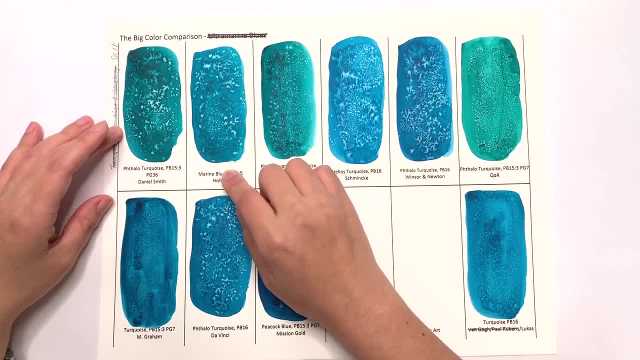 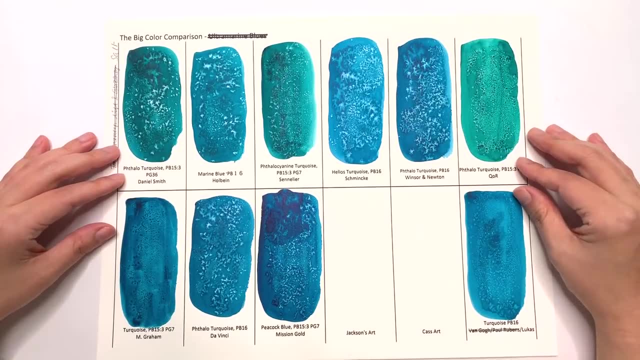 The most reactive, I would say, is the Daniel Smith, one Holbein's, one Schmincke's, one, Da Vinci and Winsor & Newton. So I would consider those colors, if you do like using salt in your painting. I'm just really. 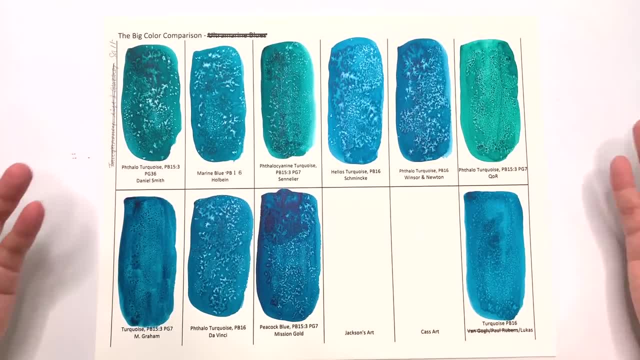 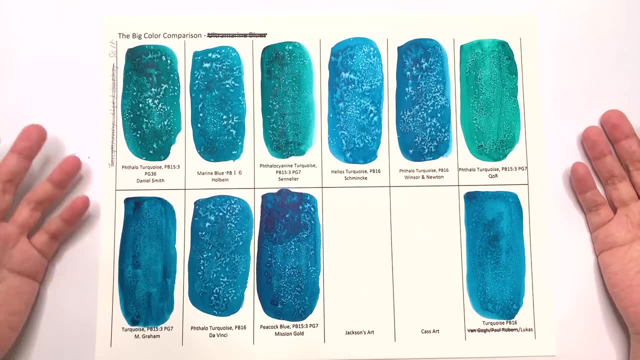 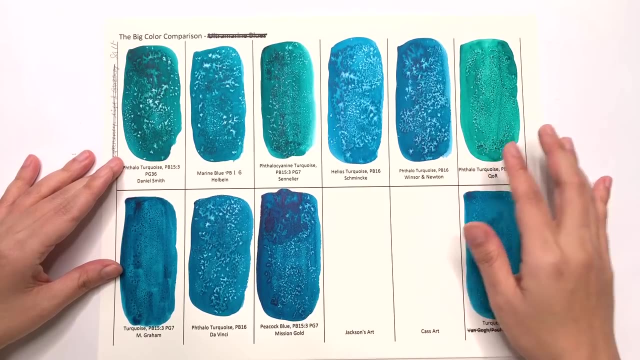 surprised again at how varied the reaction to salt or the colors have been, And it'd be very interesting to see if this will continue throughout the series. And I don't usually have a good word to say about Winsor & Newton personally, but I have to say I do like the pattern. 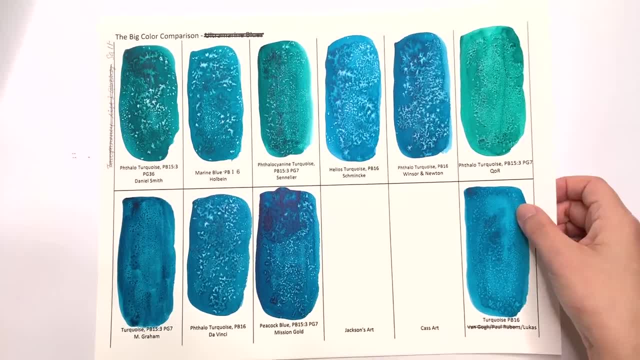 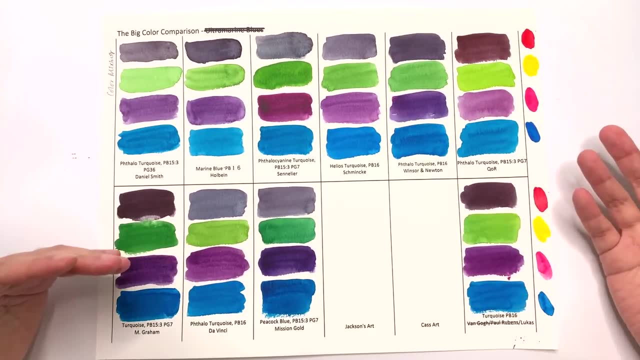 that this one created. It's really, really nice. And then, finally, we take a look at the color mixes. I said in the last episode that doing 12 color mixes for all the colors kind of nearly drove me mad. So, with suggestions from my dear patrons, we've. 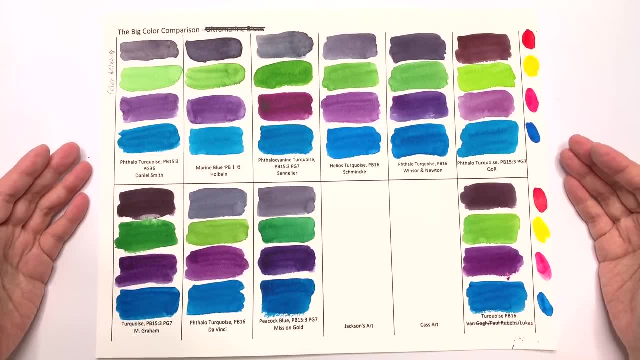 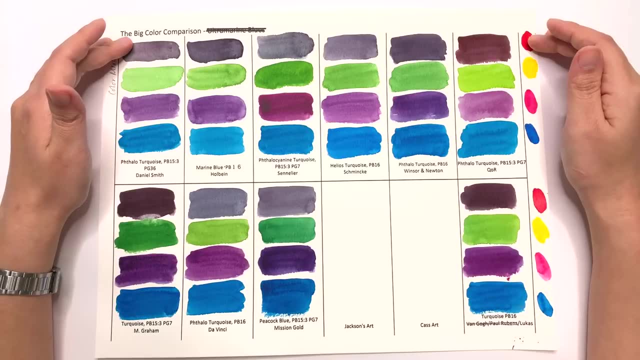 taken down the number of colors to four colors. We're going to be mixing each episode's color with its own color. So I'm going to be mixing each episode's color with its own color, So I'm going to. It's complimentary In this case for phthalo turquoise. it is a warm red, So here I'm using. 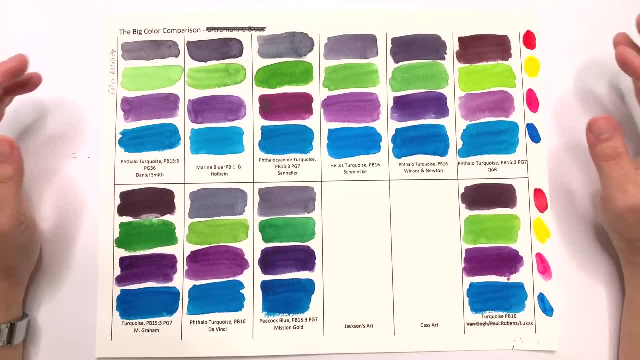 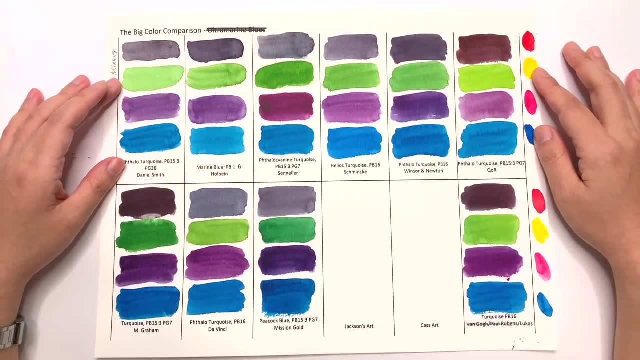 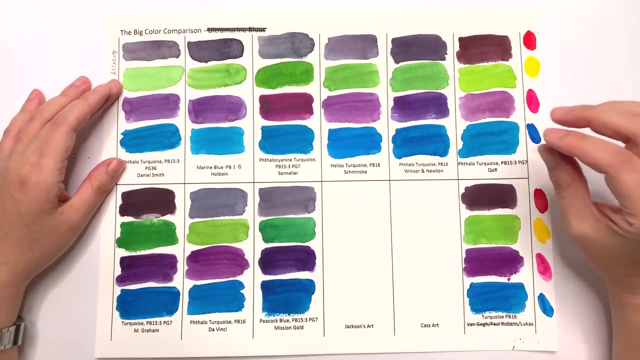 Permanent Red by Daniel Smith, And then we're going to mix with three primary colors And for that I did choose the CMY colors rather than red, yellow and blue, And the reason for that is the queens and the phthalo really helped me in the last episode to see how weak or strong a particular 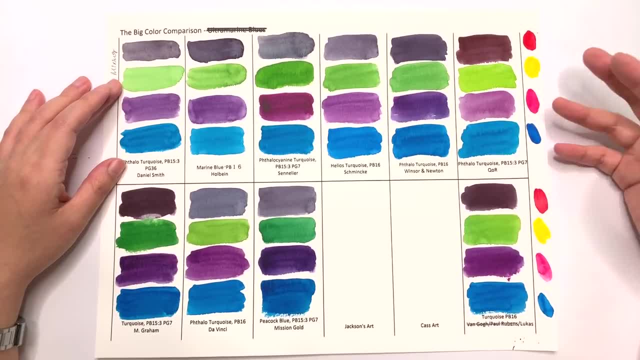 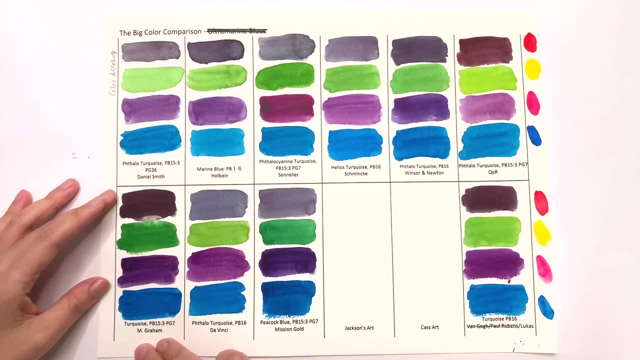 color's tinting strength was, Whereas colors for red, yellow and blue don't tend to tell me that information quite as much. and in terms of the highest tinting strength I would say M Graham wins out. It had really really strong tinting strength In second place. 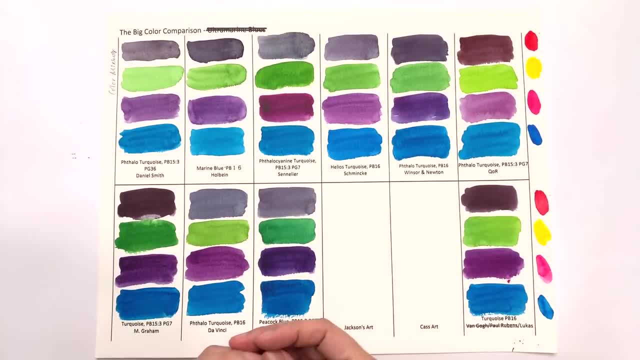 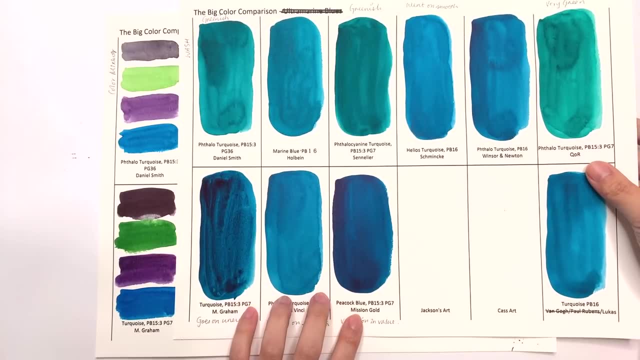 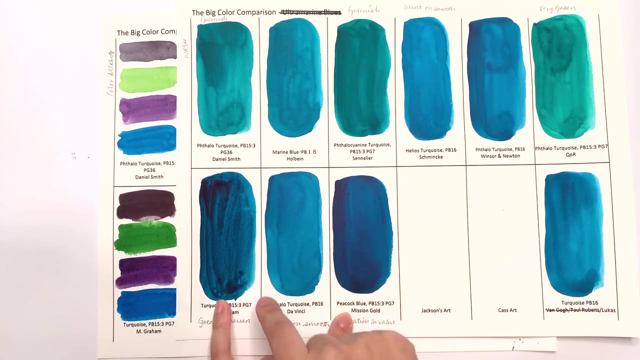 I would say it's Mission Gold. So it's really interesting that the two brands that we kind of saw as most uneven- as we saw in the main swatching, these two were kind of more uneven than, say, like DaVinci one there's a lot more dark patches than all the other colors. It's interesting that those 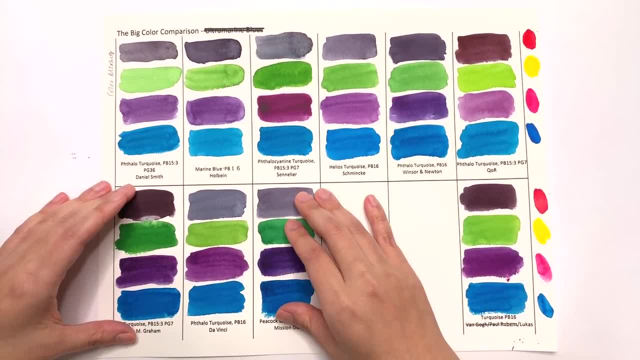 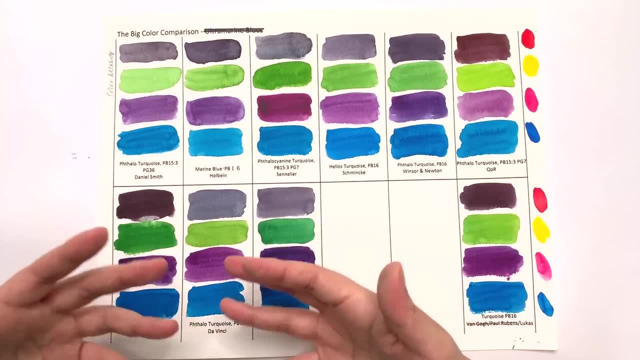 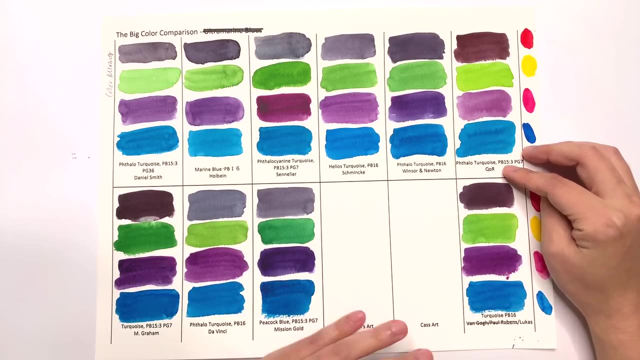 two brands also happen to be the most highly tinting strengthened colors, and that kind of makes sense. It's because they have such high tinting strength and have darker patches. When we looked at Core, we said that it was really green compared to the other colors, and that really does. 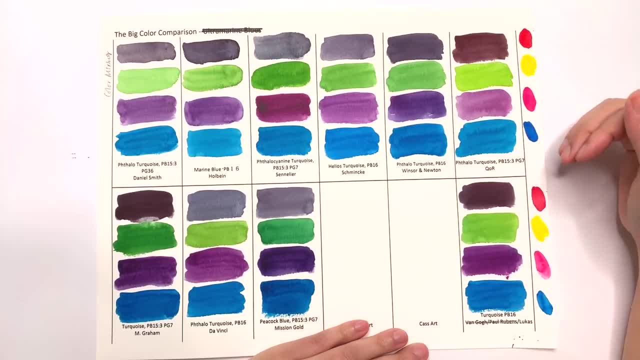 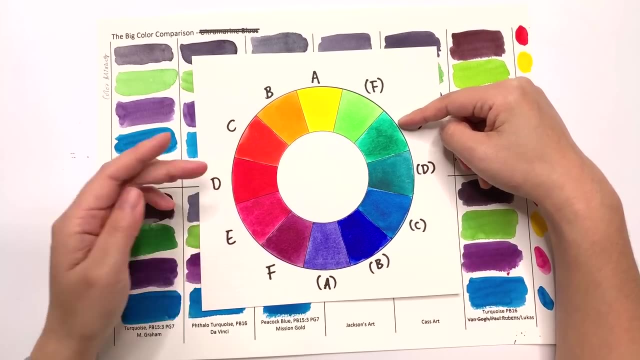 show up in the color mixes because it's more towards the green. The complementary color needs to be a little bit of a cooler red than the permanent red. This is Phthalo Turquoise being a lot more green. so let's say we're over here. Its complementary color needs. 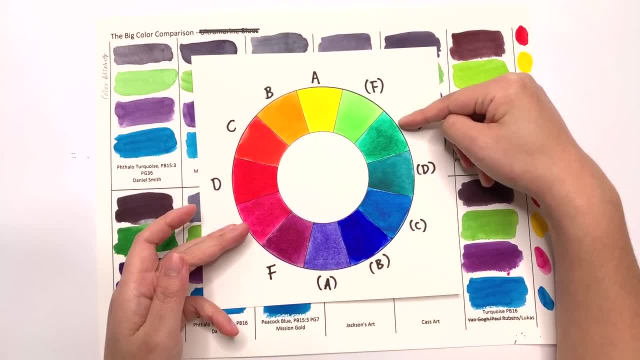 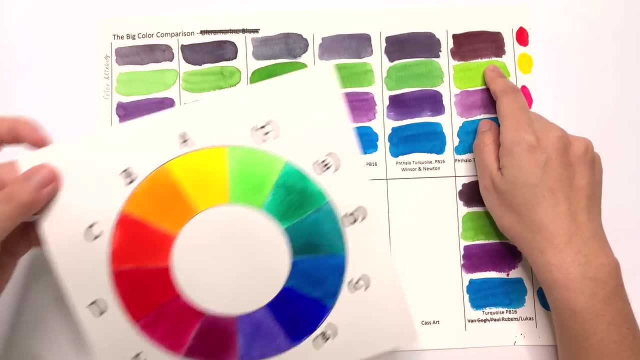 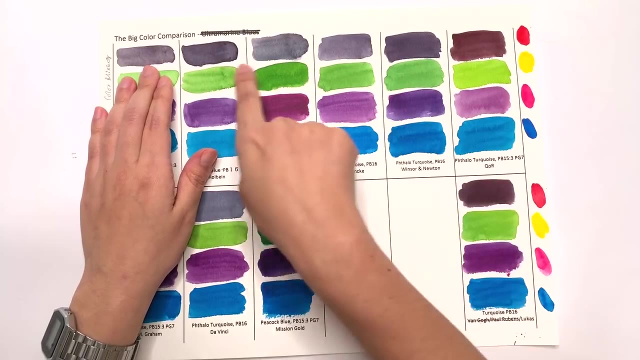 to also come down. so really the complementary color to the Core one should be more like a Quinacridone Rose rather than permanent red. and that really shows up here in the neutralization line, in that this is not quite as well neutralized As these ones. there's too much red in here, not enough blue, and you can see in the three color. 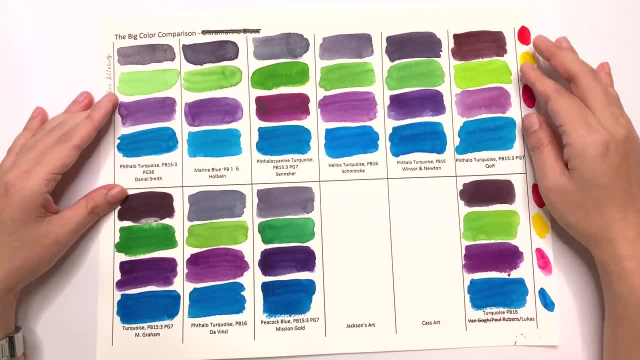 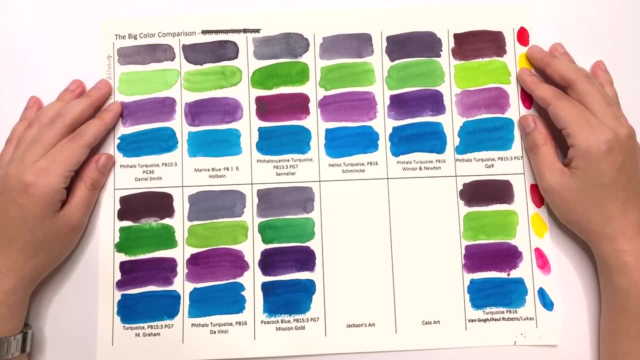 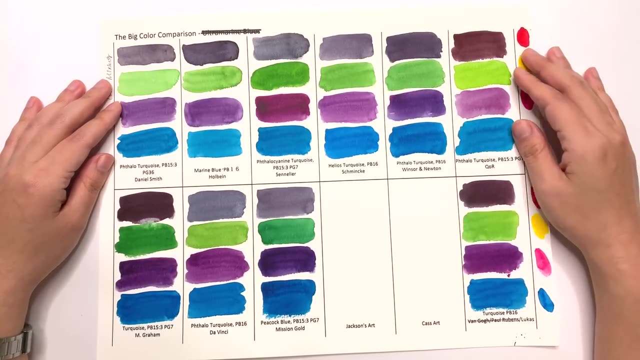 mixes of the primaries that it's slightly different color from the rest. so with the Core one, I would personally say that it's a very unpredictable color. it's a lot greener than certainly I expected and it mixes differently to a color that is called Phthalo Turquoise. 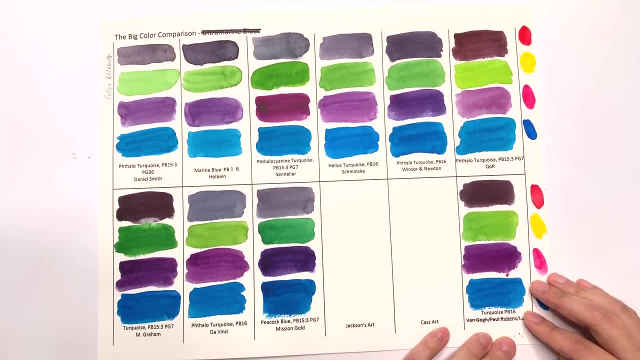 Another surprise was the Lucases one. I would have thought, it being full of fillers and things, that the colors would be really not nice. but I don't hate these colors, I think they're fine, so that's a surprise to me. I really would have thought that. 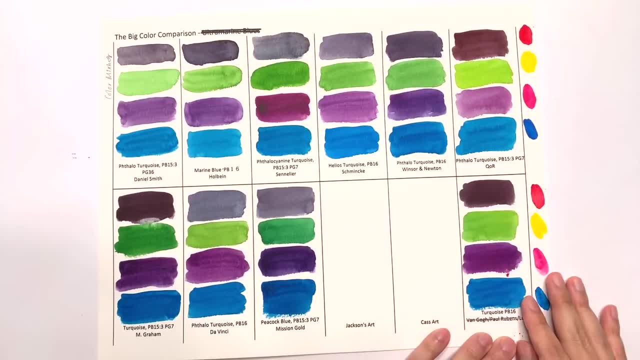 the colors would be more chalky and horrible. In this comparison it's not that bad, I have to admit. I wouldn't say it's as good as the rest, but it's also not as bad as I would have thought a color with a filler would perform. So that was all the tests we did. 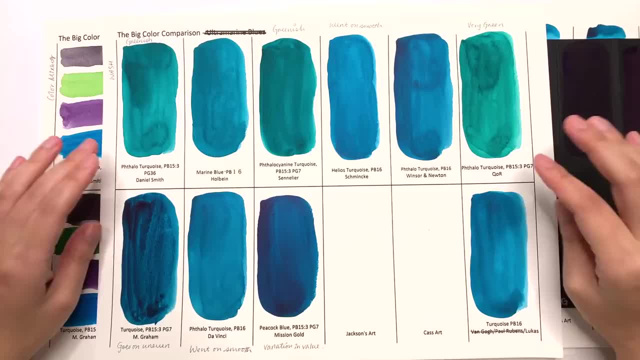 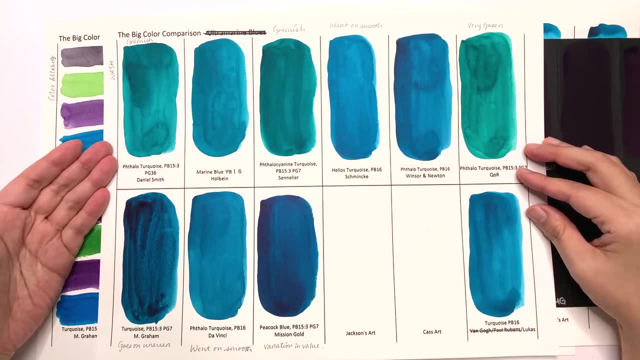 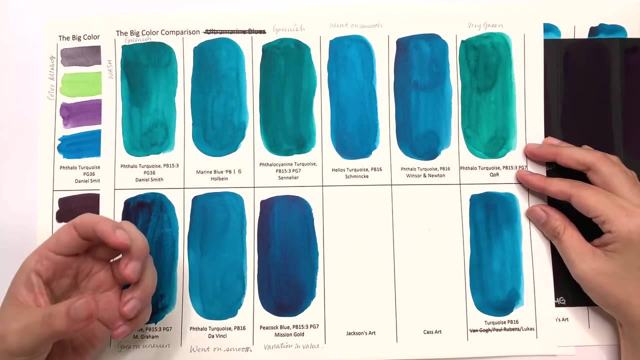 and we compared the Phthalo Turquoises. Which one is your favorite? I still really like the Daniel Smith one, but I do tip my hats off to Da Vinci for creating a very smooth color that is also very good at doing gradated washes. I am very impressed by Da Vinci's work and maybe once I 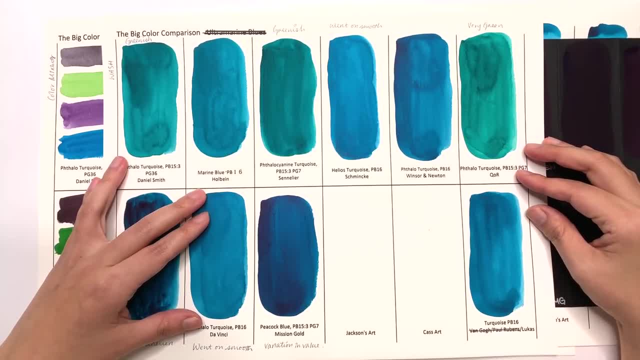 run out of all my mini tubes of Phthalo Turquoise by Daniel Smith that I have, I might move on to the Da Vinci's one. The one that I was least impressed with won't surprise you: it is the Coors one. It's just too green and it behaves in such an odd way, and there's don't seem to be any other quality.